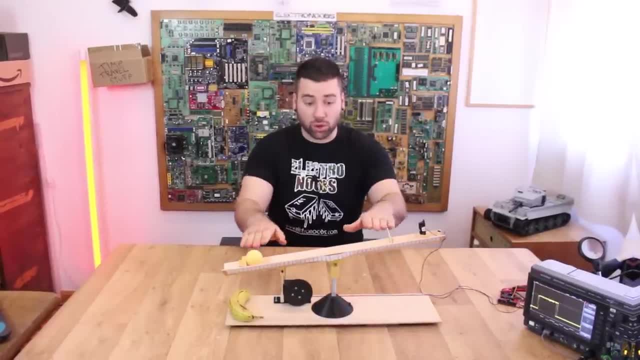 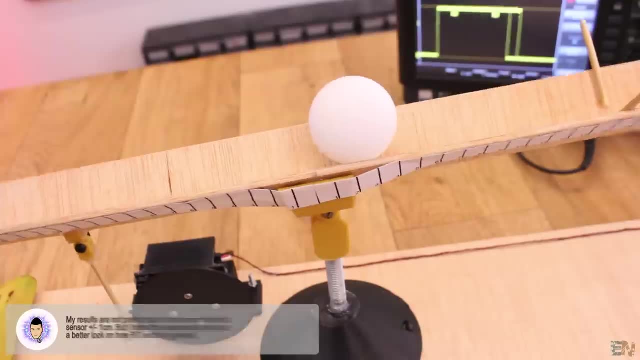 have a servo motor that will move the bar up and down and, by that, control the position of the ball. So all we have to do is apply the PAD control and react to the speed and to the position of the ball and keep this ping pong ball always in the middle. Everything is controlled with an Arduino that will 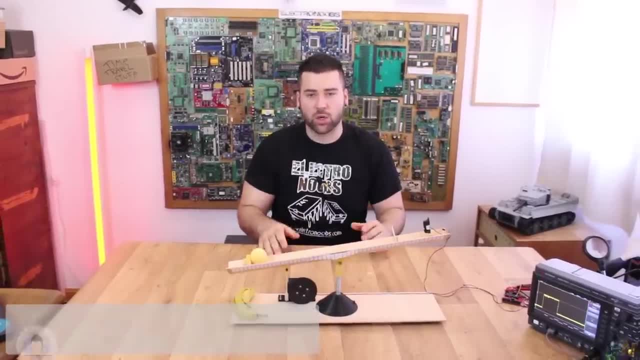 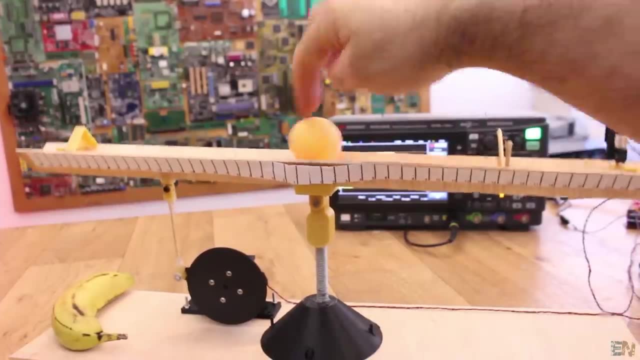 measure the distance to the ball and also control the servo motor. So it is pretty obvious that if the ball is a little bit more to the right, the bar will move and push the ball to the left, And if the ball is a little bit more to the left, it will do just the opposite. Okay, just let me show. 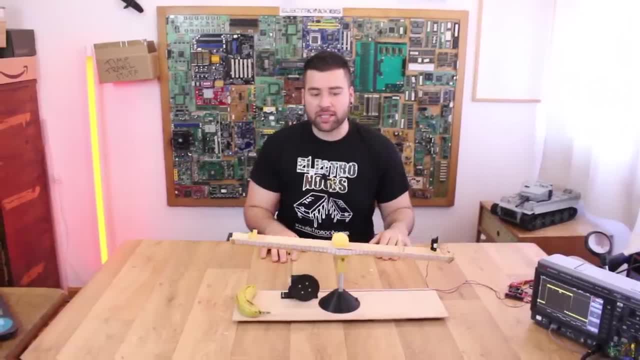 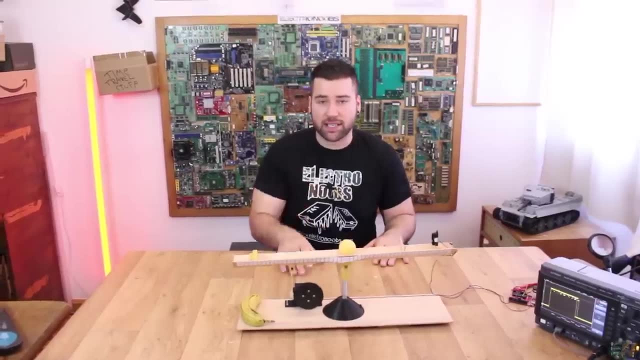 you a quick example: I'm powering the power supply and, as you can see, the ball should stop exactly in the middle, pretty much in the middle, And this will oscillate a little bit because the sensor that I'm using is not very precise and will have a little bit of error. So let me just stop this. 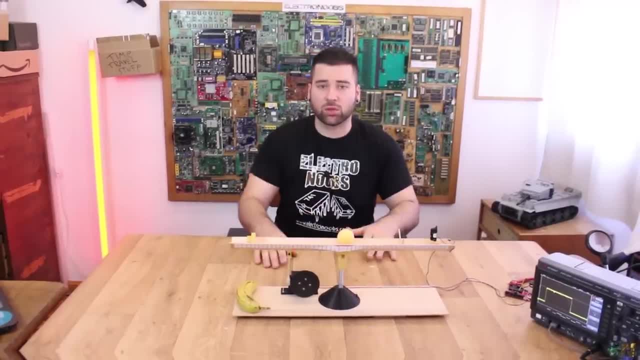 because it makes a lot of noise. The idea goes like this: we have to use PAD control to keep the ball exactly in the middle. So in this video, I will show you how the same thing. I will show you how the same thing: you can control the simulder to keep the ball exactly in the middle. So in this video, I will show you how the 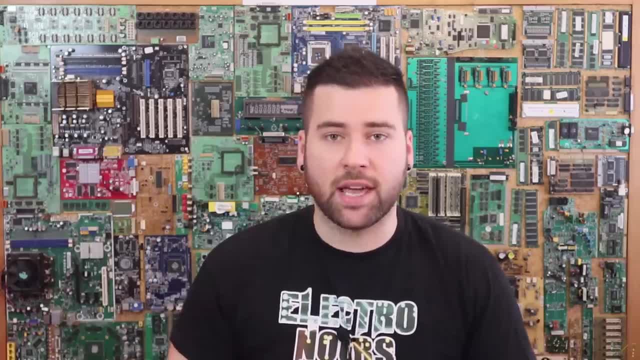 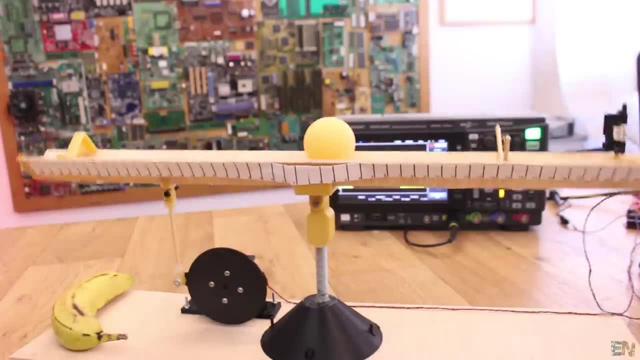 the works, how to build it, and we will also make a lot of tests and try different values for the PID constants And finally we will merge everything together into a PID control. I will try to explain the best that I can how to tune the PID constants And, once you know, how to set up this example. 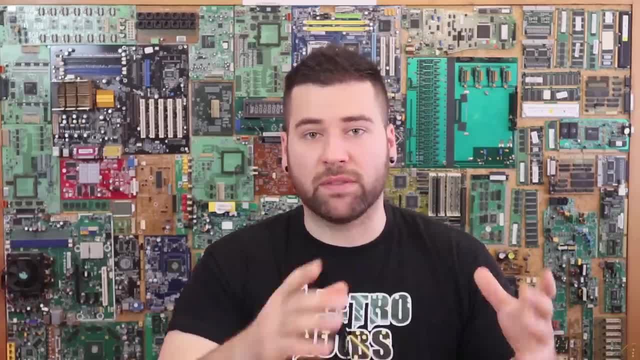 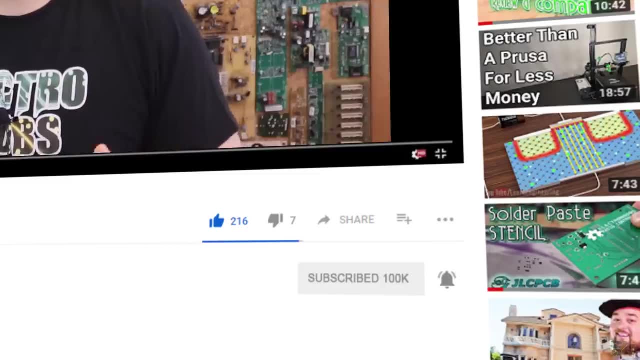 you could apply this same theory to any kind of PID control. But before you start, make sure that you hit the subscribe button but also that notification bell, because otherwise you might miss my future videos. The notifications distance for the YouTube videos changed a little bit in the 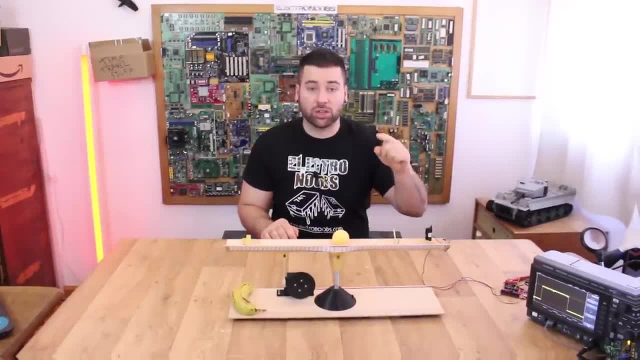 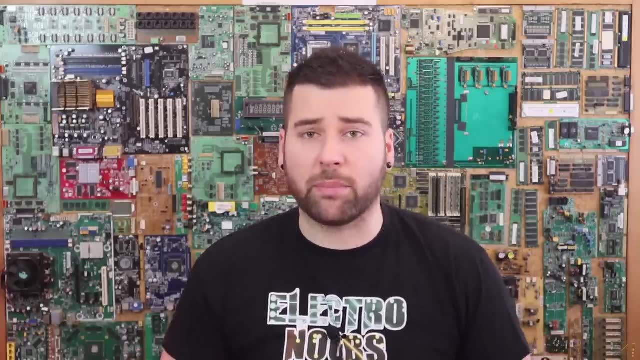 last few months. so make sure that you activate the notification bell, but also that you enable notifications in your device, and in that way, you will be able to see my videos when I post them. And, as always, a huge thank you to all my patrons for supporting my work. So let's get started. 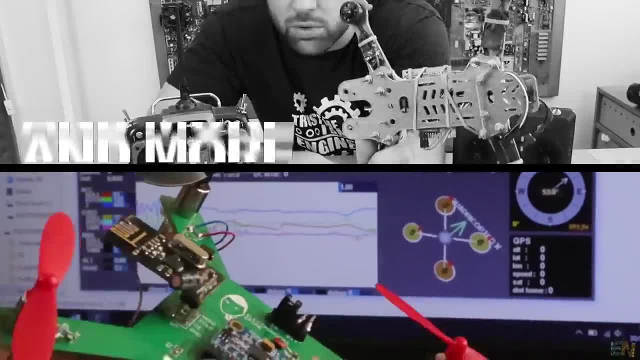 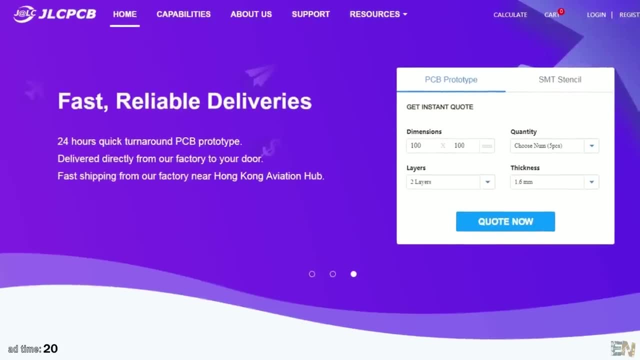 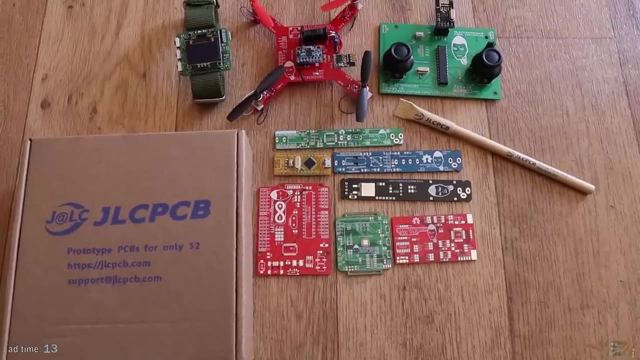 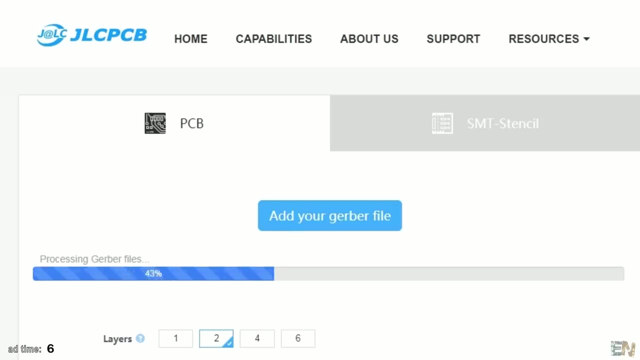 JLCPCB is sponsoring this video. They provide fast and best value prototyping services With their online and instant quote, fast fabrication and competitive prices. you can save a lot of time and money. So quote now. upload the gerbil files of your PCB. 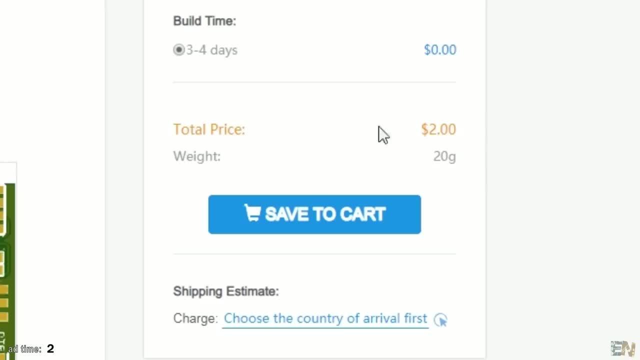 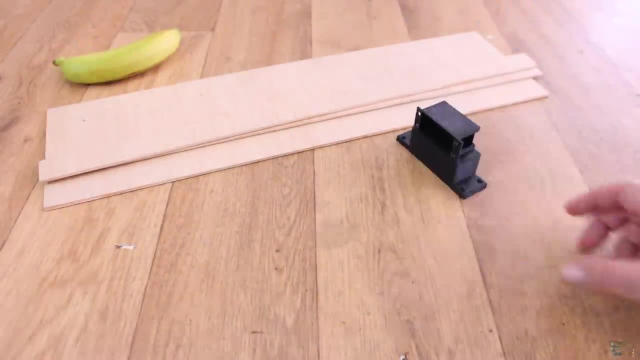 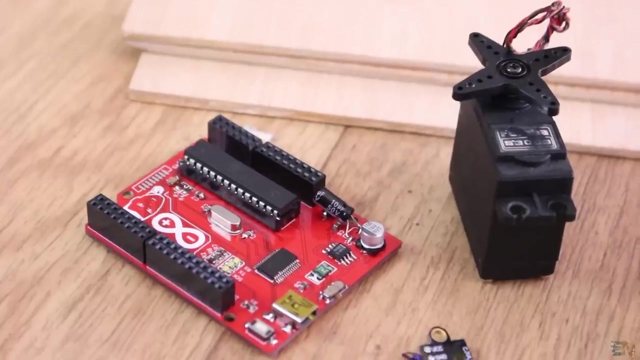 and for only $2 plus shipping, you can order PCBs in less than 5 minutes. What's up, my friends, welcome back. Let's start by building the balance first. This will be very easy and very fast. If you want to make this same experiment and learn how this works, you will have the 3D files. 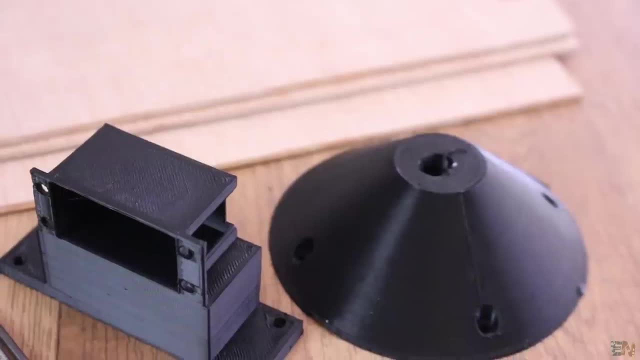 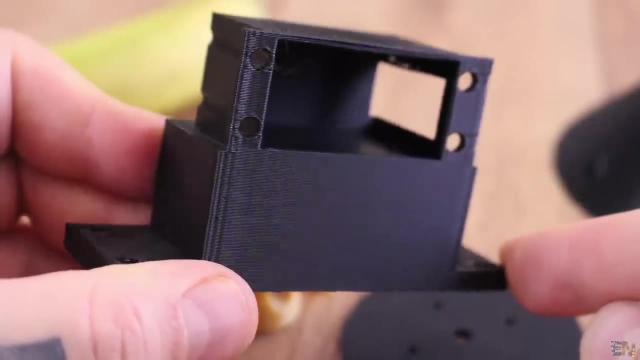 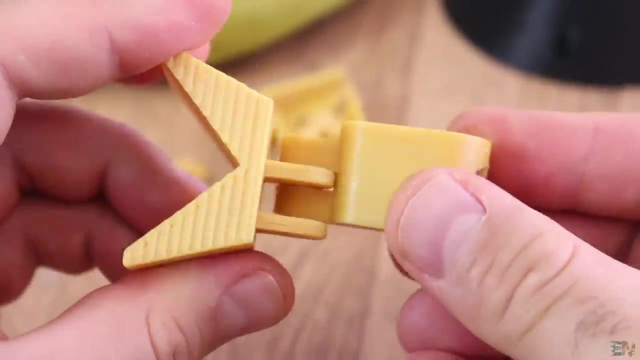 for the balance below this video, Print the parts with PLA material, 0.4mm nozzle and 0.2mm layer height. We have this main support. Then we have some small parts that will create some sort of hinge that could move left and right. We have this support for Futaba servo motor. 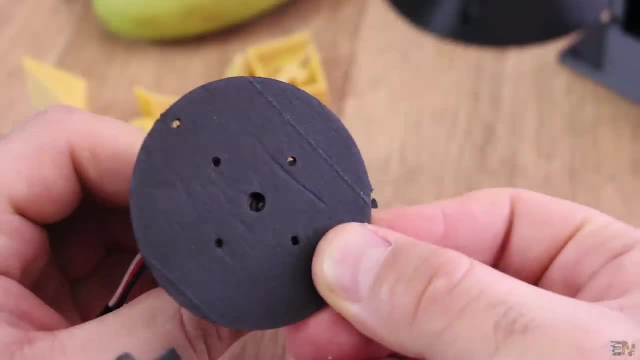 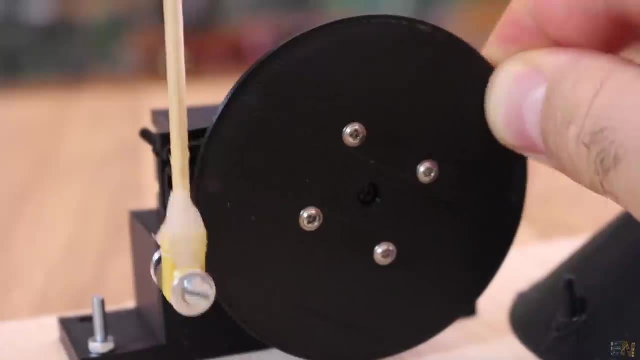 and we also have a disk that will be connected to the shaft of this motor. Then we have this small parts that will be used to transfer the movement from the servo motor to the balance. We also have this plastic endstops that will be used later. 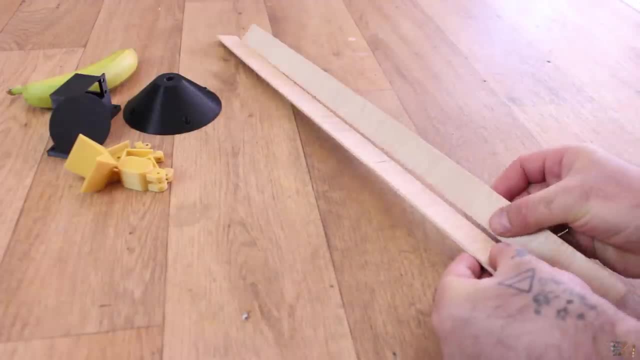 For the moving rail. I will be using some plywood parts, Because printing parts this big will take a certain amount of time. The میں will be a little bigger than the service table. I will also use a small piece of bevel to shape the flavor. I will use a few wood pieces. I will also use a little wood of metal. 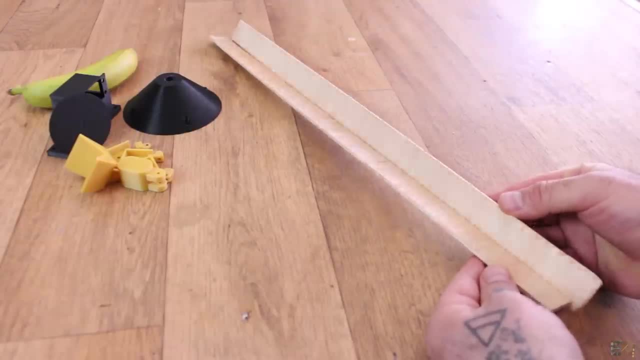 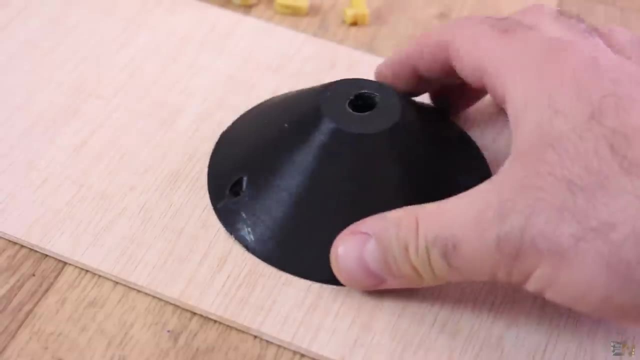 I will glue these two parts one to each other with a 90 degrees in between, and then the ping pong ball will be able to roll on this groove. I will screw the entire balance to another piece of plywood, and that's it for the body of this project. 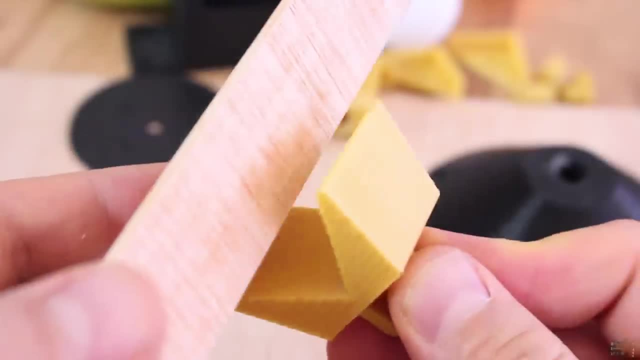 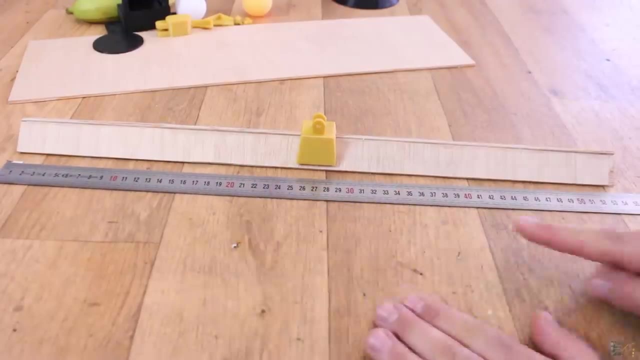 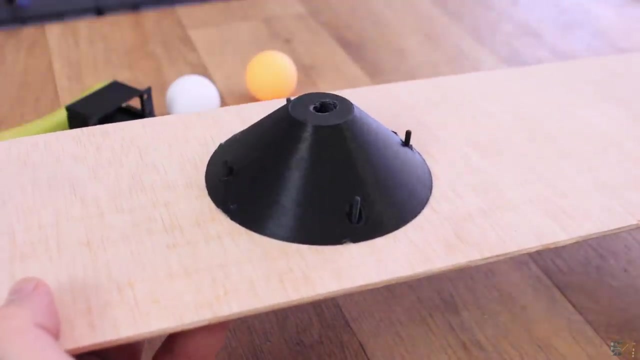 So once the glue for the long plywood part is dry, I glue that to this plastic part and make sure that the part is exactly in the middle, so the balance will rotate with the same force to each side. Then I screw the main base to the other plywood part using some entry screws. 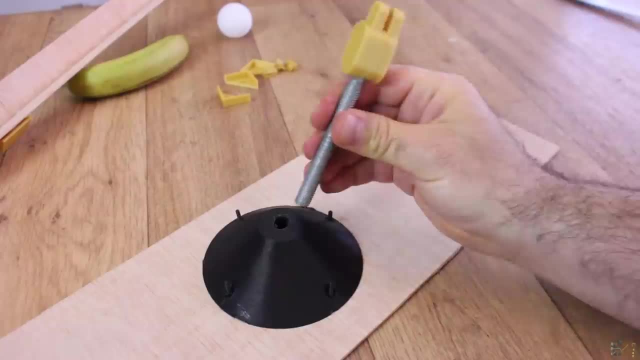 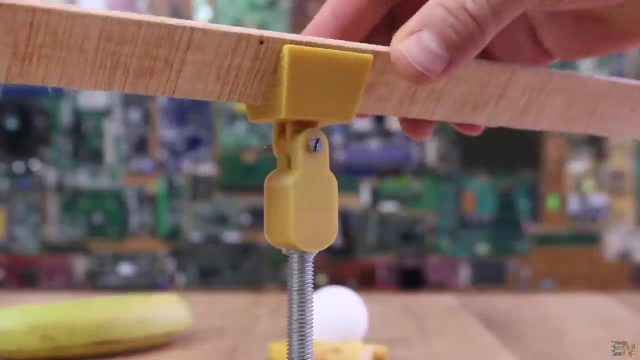 Now I add a short 8mm screw to this other part. Now, on top of this support, I add the balance. I place a 3mm screw and I make sure it could rotate with low friction right and left. so now the main body of the balance is ready. 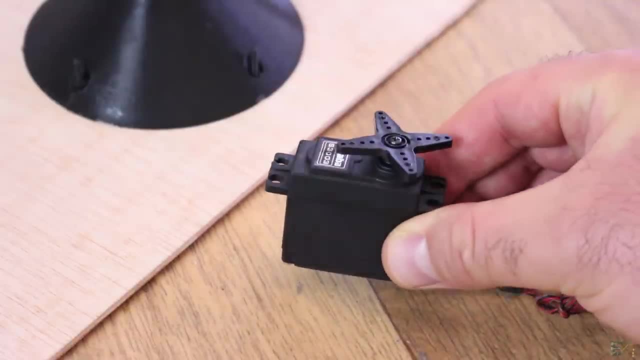 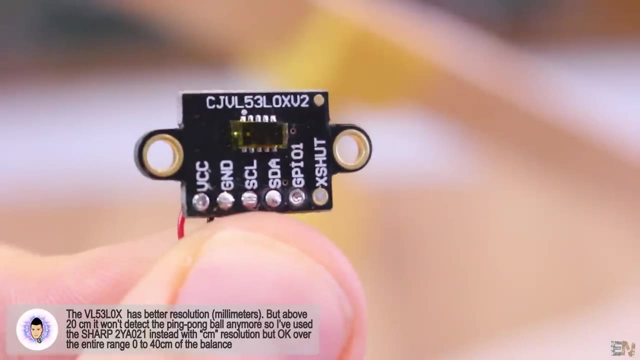 To control the movement I use the S30-03 Futaba servo motor and to measure the distance I first wanted to use the S30-03 Futaba servo motor. I used the VL53 L0x laser distance sensor, but that wasn't precise enough for distances. 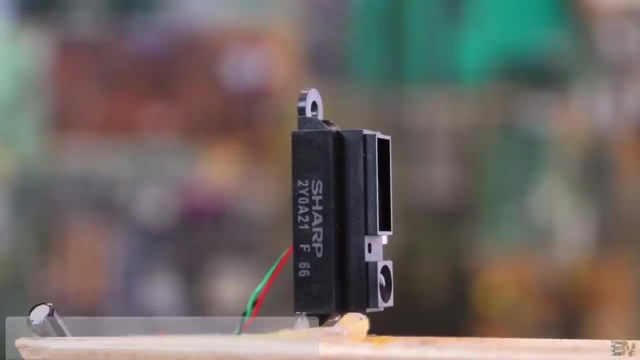 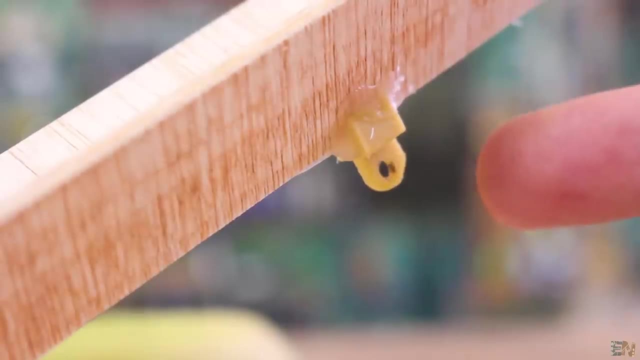 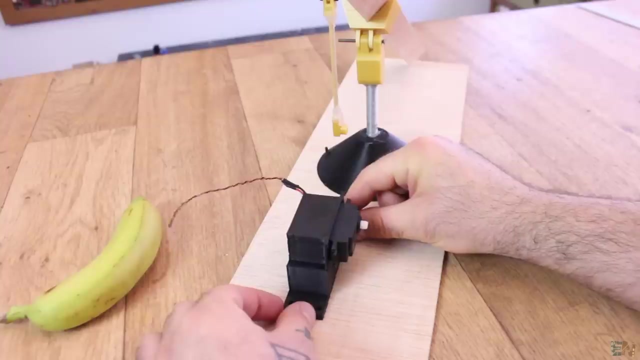 above 20cm. That's why I've used another infrared sensor, the Sharp 2Y0821.. So I glue the other small parts to one side of the balance. Now I make this other part with a wood barbecue stick in between. 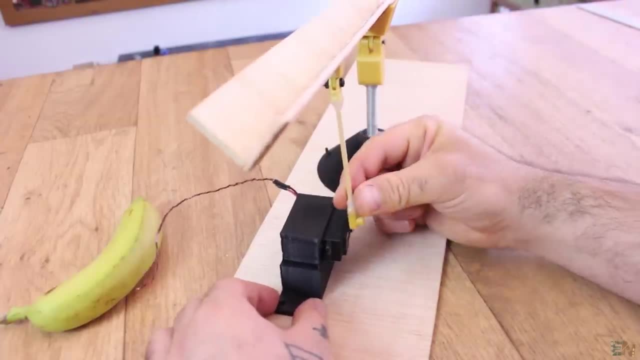 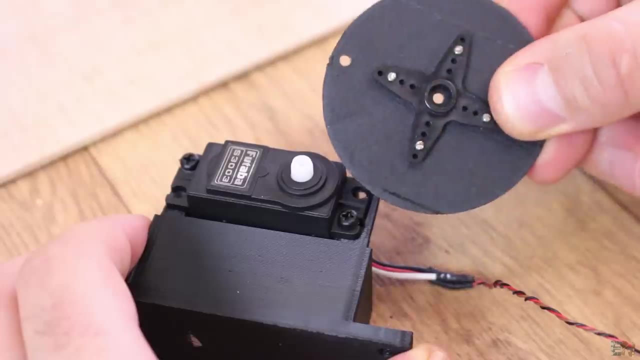 I measure more or less where to place the servo support. Now I add the servo motor to that support. I place the servo motor on the side of the balance. I screw that in place Now I put the servo in the 0 degrees position and I add the disc using the given star shaped. 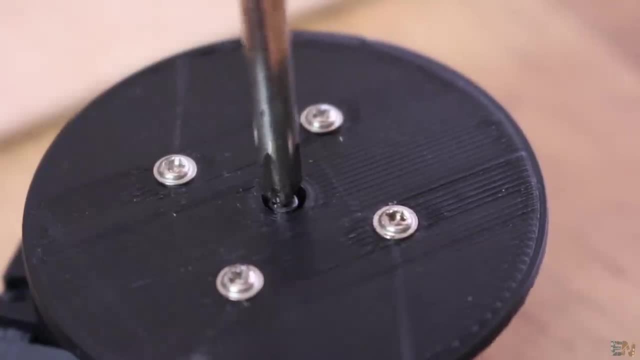 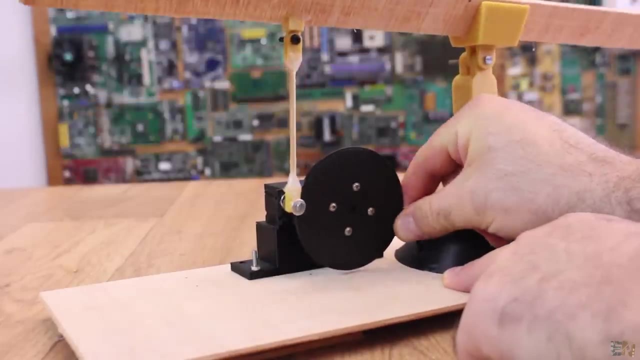 part from the servo and I tie the screw. Now I screw the support in place and connect that to the balance. Now it will move up and down and by that it will change the angle of the balance. Below you will find some different sizes for the disc, in case that you need faster or slower. 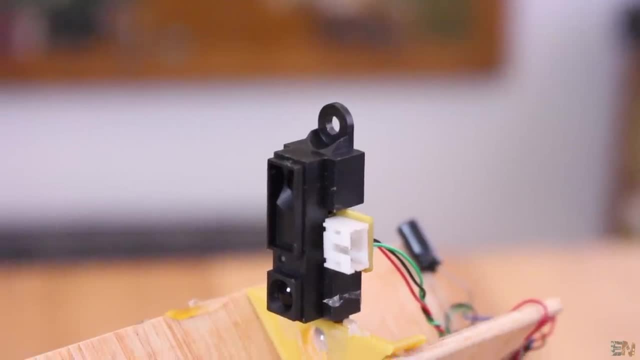 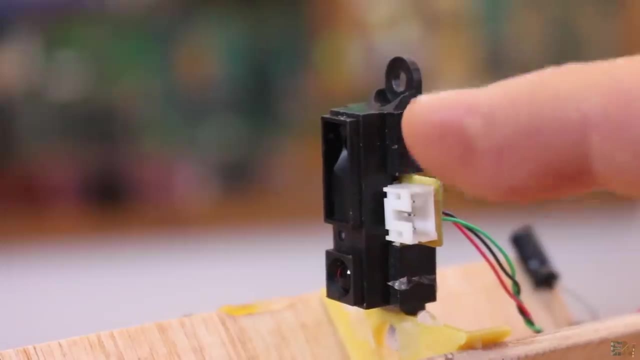 movement And for the infrared sensor again, I will finally use the Sharp 2Y0821.. I screw that in place. I screw the servo to the other side of the balance. The other sensor lost a good resolution over 20 cm. 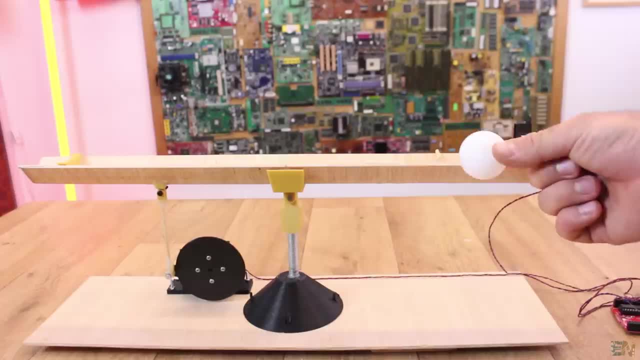 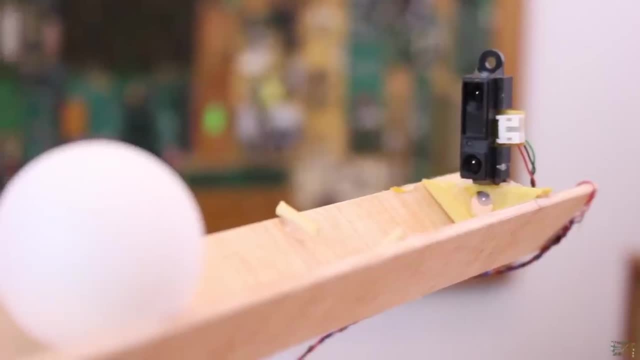 This one has a lower resolution but is kind of the same over the entire range from 0 to around 40 cm. So I glue the sensor to one end of the balance. I also add a 10uF capacitor as a filter at the sensor output. 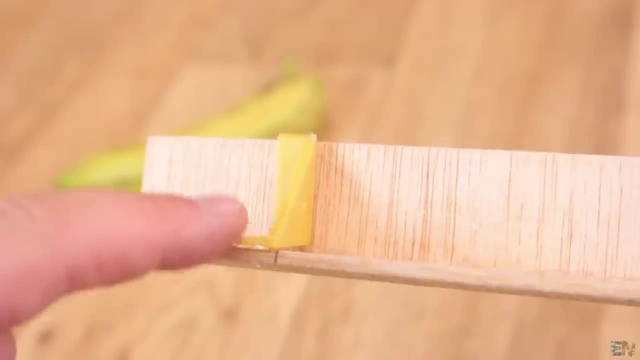 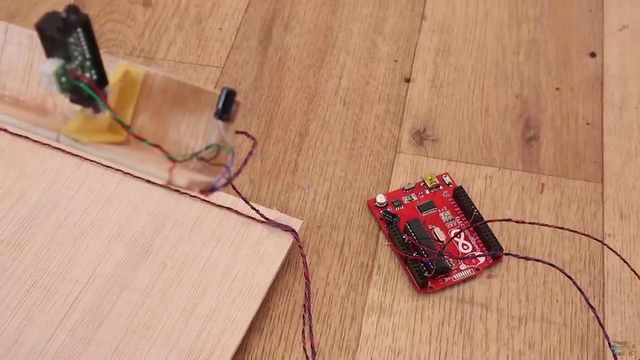 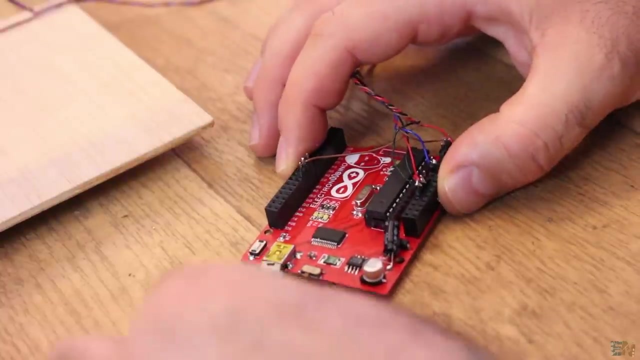 So set the schematic for more. I place another end stop to the other side. Now I pass all the other sensors, Now I pass all the wires and connect those to the Arduino. that will be placed here and the setup is ready for tests. Check the schematic for this below and also the final code Download. 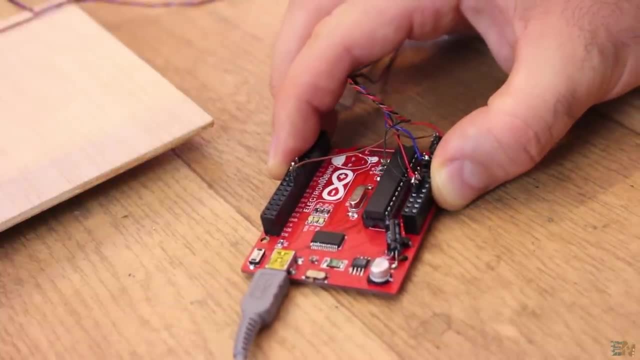 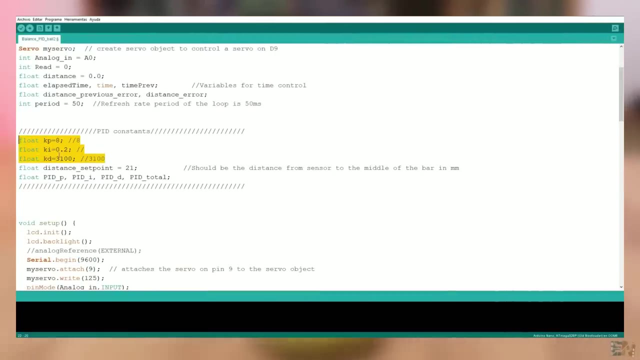 that code and upload it to the Arduino and let's start with the tests. In the code on this part you will see the KP, the KI and the KV and you could change these PID constants if you want, and try some different values Any PID system will need. 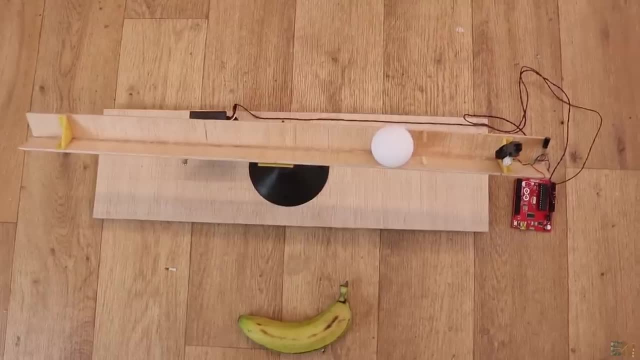 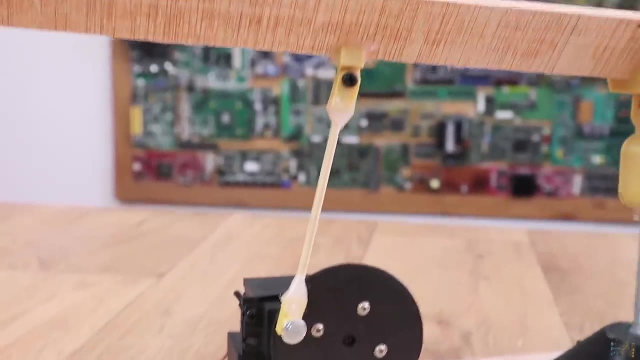 3 main parts. First, we need a feedback, which in this case is given by the distance sensor. Then we need an actuator that will change the system output, and in this case that will be the servo motor. Finally, we will need a PID code in between with a set. 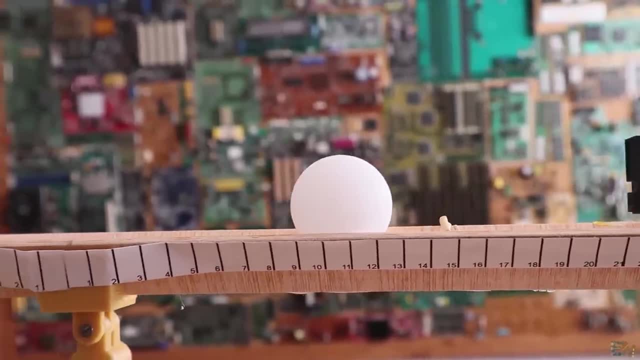 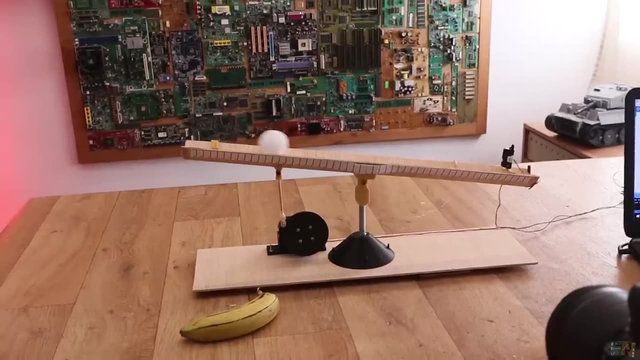 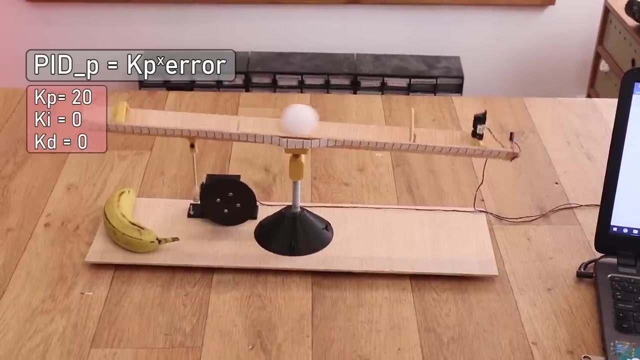 point. and that set point in this case will be the middle position of the balance. so when we measure the distance it will be half of the balance length. First we have to see the proportional action. For that I put the KP equal to a value and I will leave the KI and KD equal to 0. Now 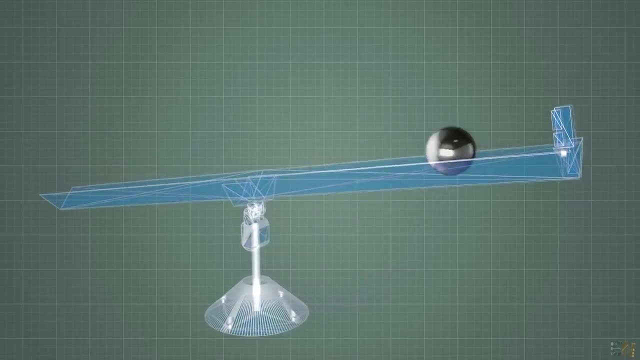 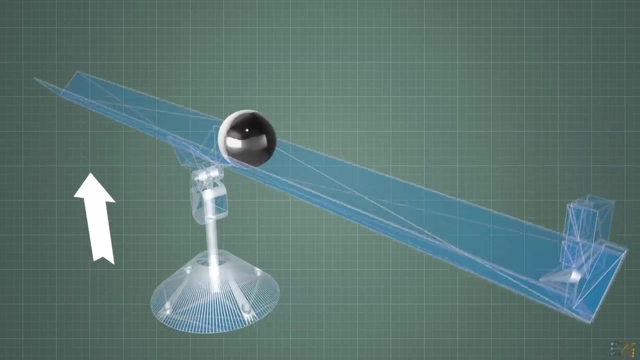 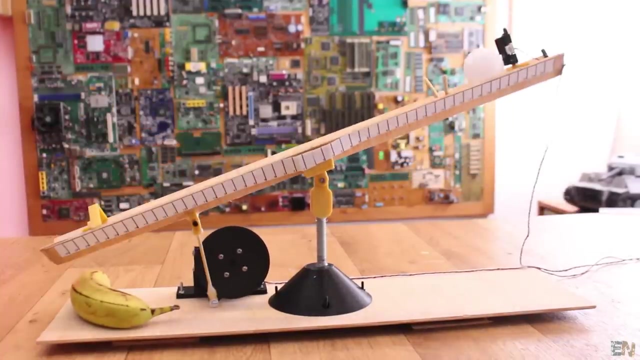 only the KP will affect the output. The sensor will measure the distance to the ball. If the distance is not 0, it will move the servo proportionally till the distance gets closer to the center. Look what happens with the KP equal to 20.. The system oscillates too. 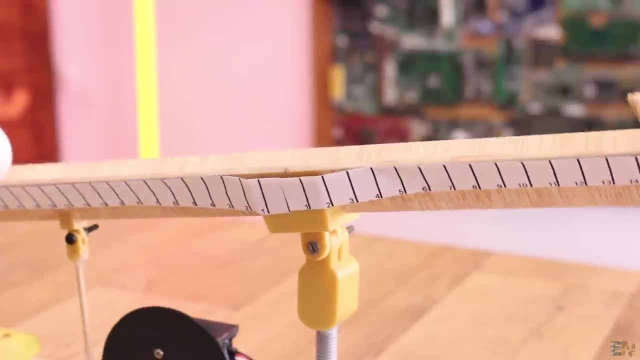 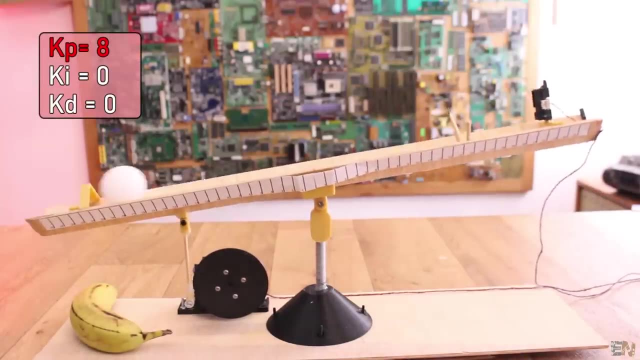 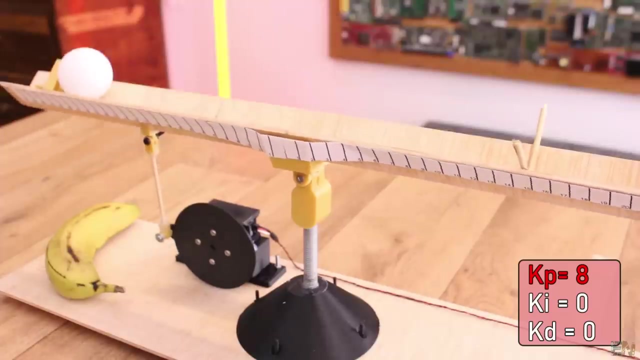 much and also too fast, so we have to put a lower value. I now make the same tests, but I lower KP equal to 8.. Now we have a pretty decent oscillation, but the ping pong ball won't stay in the middle, and that's pretty obvious. If the distance is too high, the balance will. 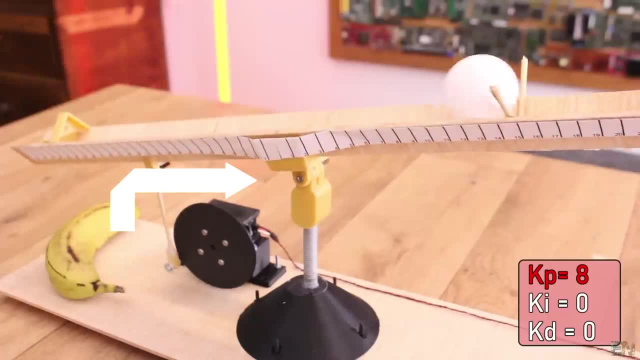 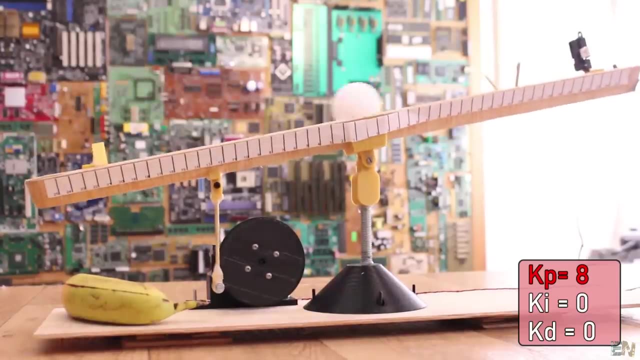 rotate clockwise, and if the distance is too low, it will rotate counter-clockwise, and that will always end up in an oscillation. but don't worry, that is good for us. All we have to do now is to measure the PID and the KD for the PID. This is what we will do. 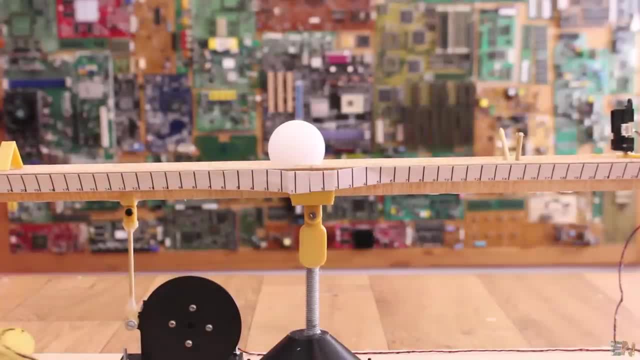 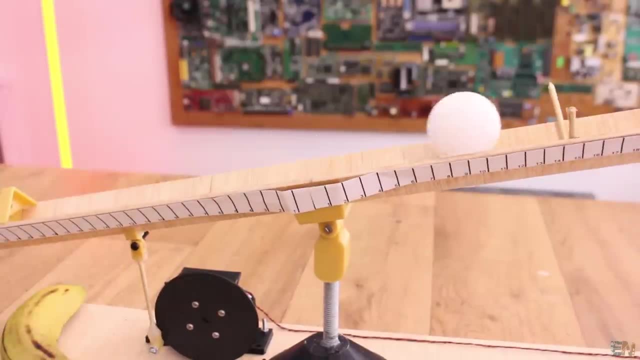 for the PID is to rapidly stop the ball when it's in the desired position. In order to make some fast changes. we have to react to the speed of the ball, not to the distance anymore, But speed is equal to the distance divided by the time. 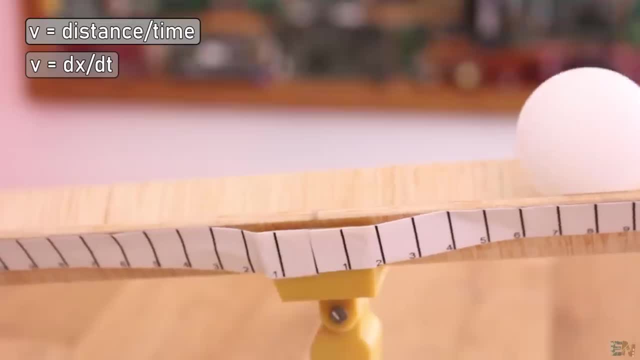 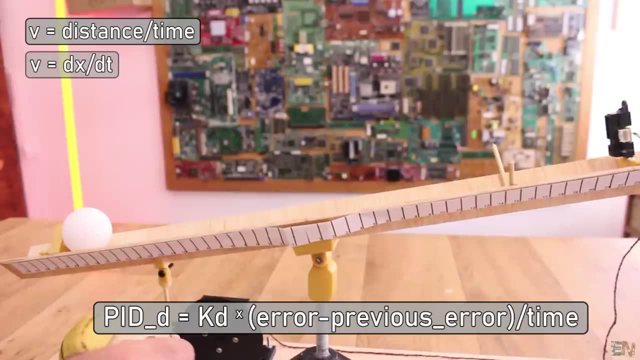 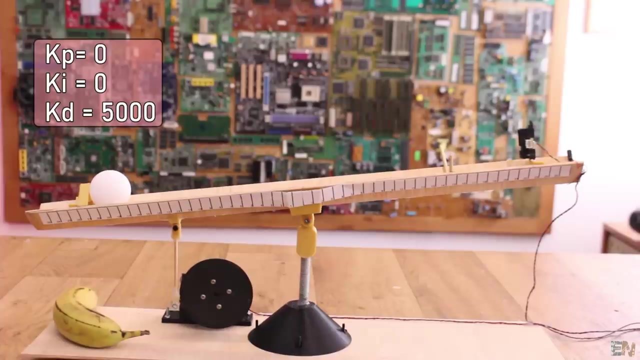 and that's delta X divided by delta T, where the X is the distance and the T is the time. So we need the derivative part of the PAD control that will have this equation. Now I put all the constants to 0, but I set the derivative part to 5000.. Now look what happens. 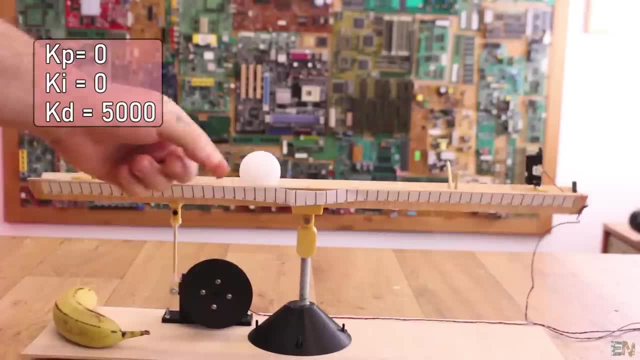 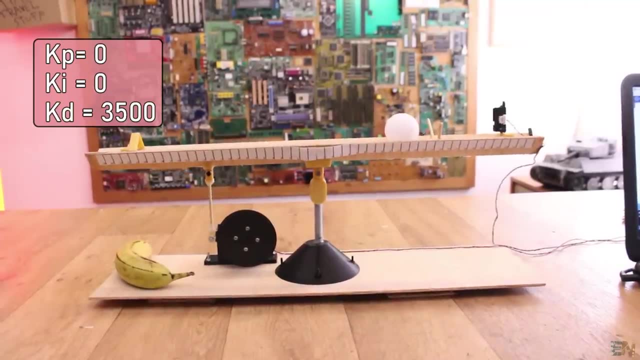 The reaction to the speed of the ball is too strong, so we have to lower the value. So now I set the KD to 3500.. As you can see, the system reacts very fast to the speed, not to the distance anymore, and by that it will stop the movement. 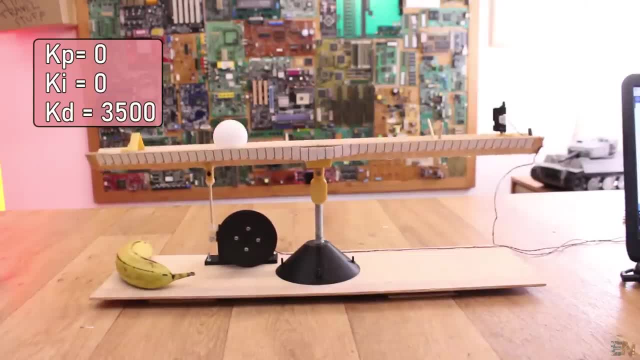 But now we have a different problem. Now the ball will stop in the direction of the PAD control. Now we have a different problem. Now the ball will stop in the direction of the PAD control. Now we have a different problem. Now the ball will stop in. 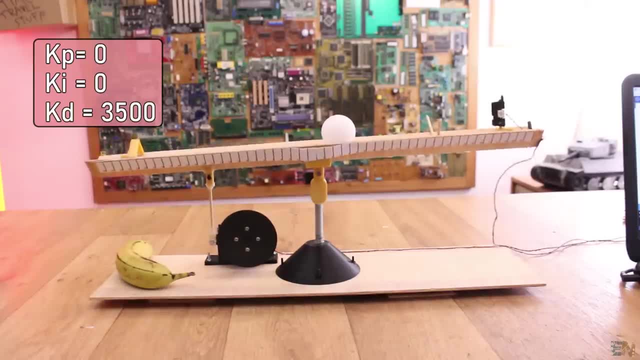 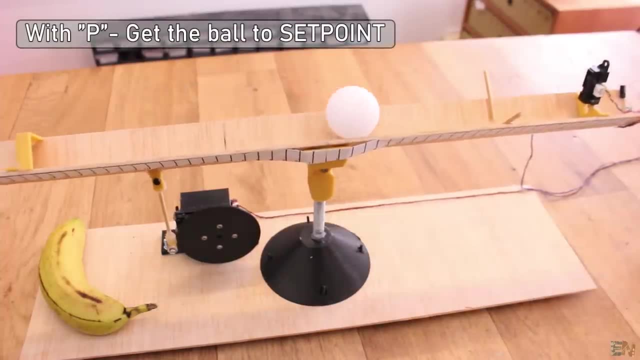 any position and we don't want that. We want it to stop exactly in the middle. So for that, before, as you remember, with the P control the ball passed in the middle each oscillation. Now with the D control we could stop the ball. So if we combine these two together, 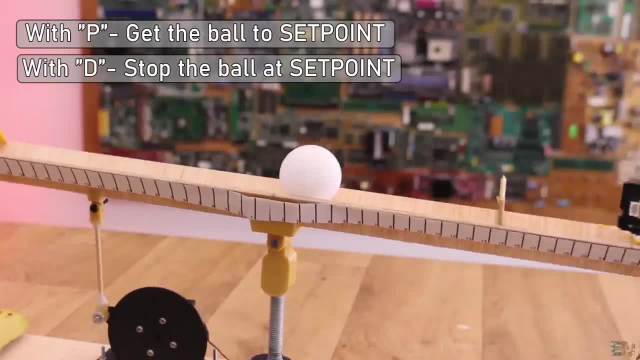 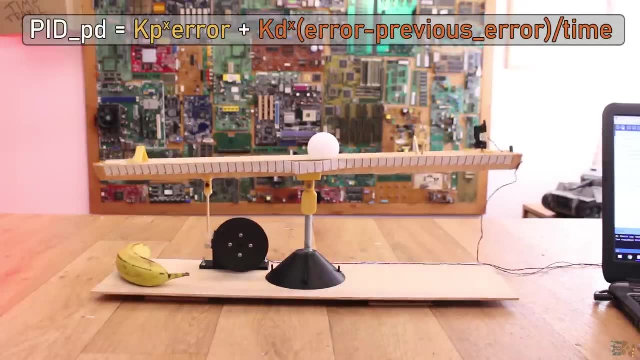 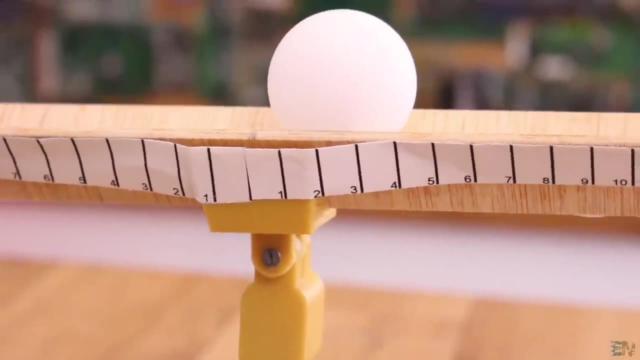 we could both stop the ball, and also exactly in the middle. I now make some more tests, but I make the sum of the P and the D constants. This is called a PD control and this is the equation. As you can see now, I stopped the ball and it is also close to the center. 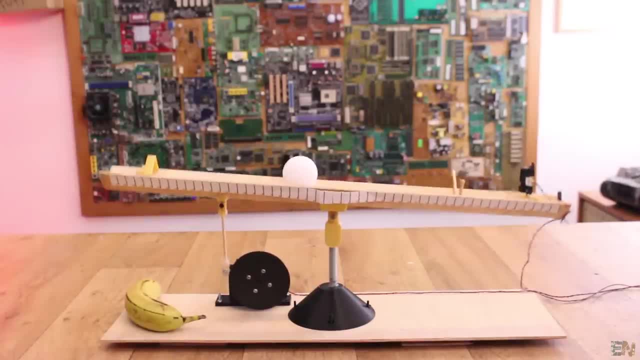 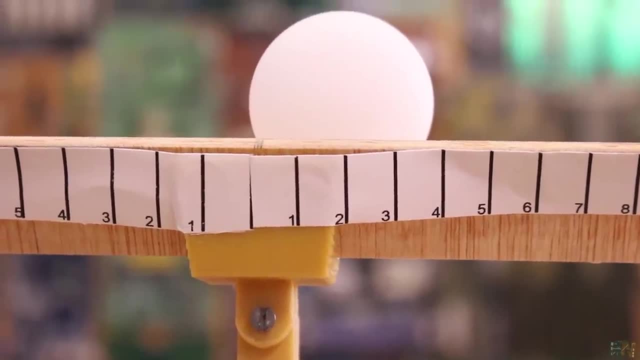 so my system works quite well for now. But what will the I variable add to the setup? Well, for example, in this scenario the ball stopped at around 1 or 2 cm, so that's not exactly in the middle. The balance isn't moving anymore. 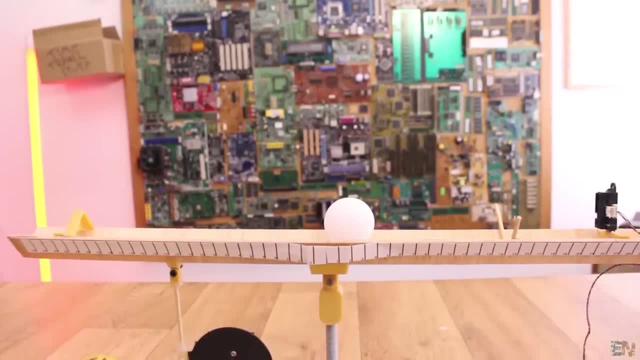 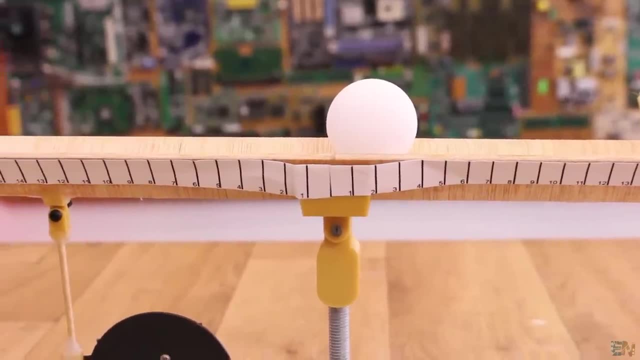 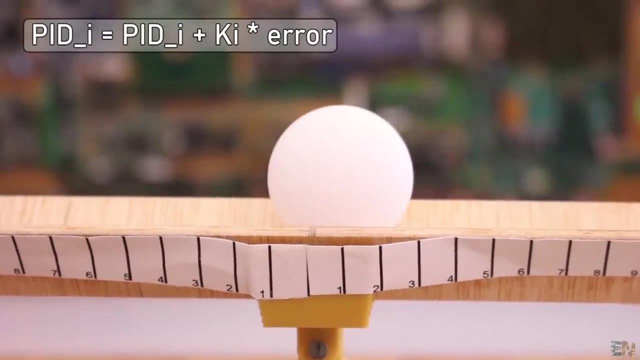 because the error is too small, so the proportional part won't affect. Also, the ball is not moving, So the speed is 0, so the derivative part won't affect either. That's why we need to add the integral. This part will sum up each loop in the code and by that will get bigger and bigger. 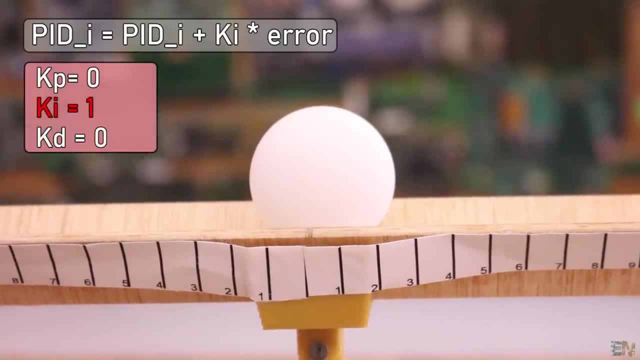 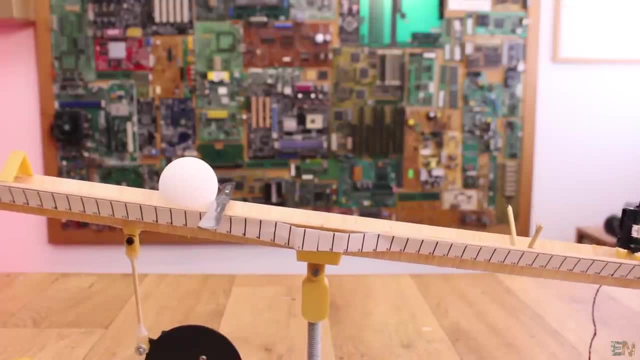 To understand better, I set all the constants to 0 and I put the integral to 1.. So now I block the ball and let's see the effect. As you can see, the more time passes, the bigger the integral part will get and the more the balance will rotate. 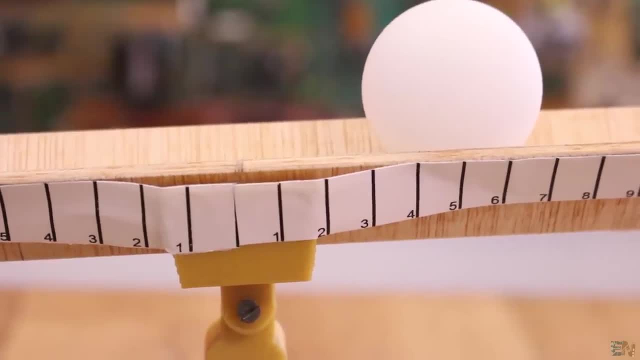 So if the ball stops at the middle, the integral will start to change. The bigger the integral part, the more the balance will rotate. So if the ball stops, the integral part will stop. So so as you can gets stuck at, for example, 2 cm, the integral part will slowly increase till the ball is. 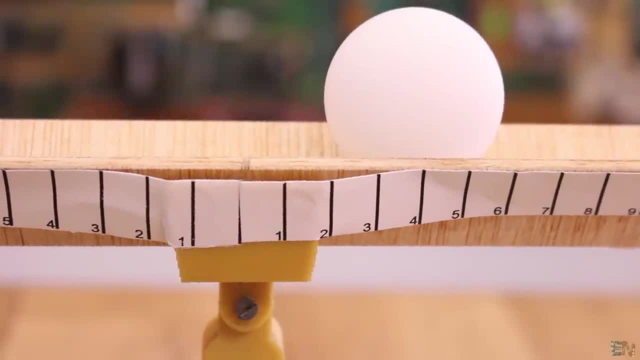 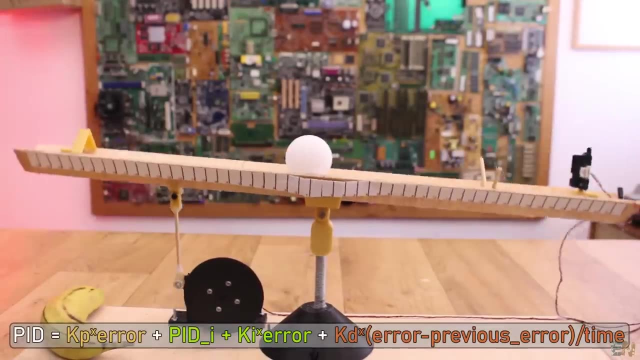 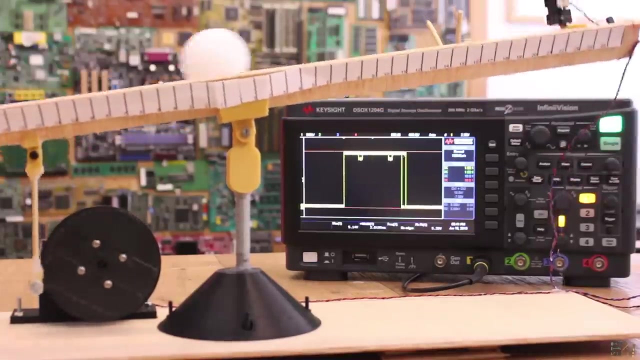 exactly in the middle. That is done very fast in the code and we will get the good PID control. So now I make the sum of all three variables. with this equation, The output of my PID control will be a PWM signal that will be applied to the servo motor and that will move from. 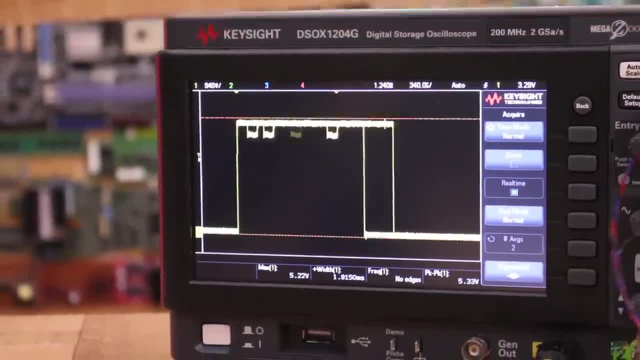 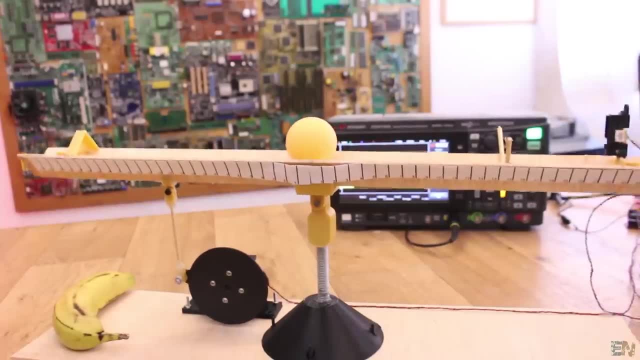 0 to 180 degrees. Now I have a pretty decent control and the ball will stop in the middle, no matter how fast I move it or from where I move it. So I hope this simple example explains how basic PID control works and why we need each.